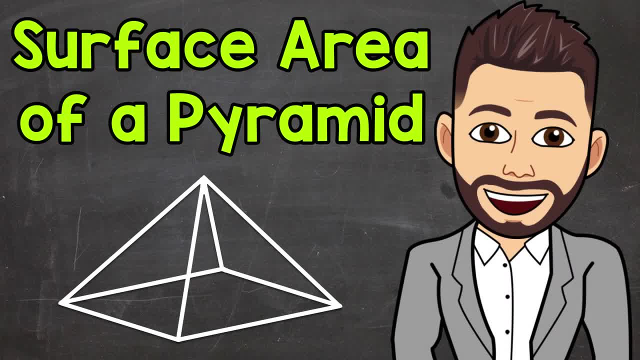 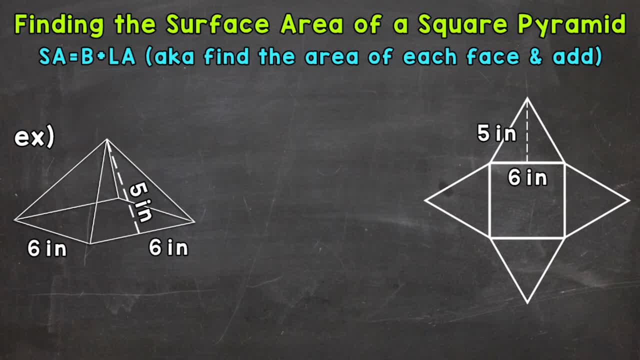 Welcome to Math with Mr J. In this video I'm going to cover how to find the surface area of a square pyramid. And remember, surface area is the total area of the outside or surface of a three-dimensional shape. When it comes to square pyramids, we have five total faces: the base and then four lateral. 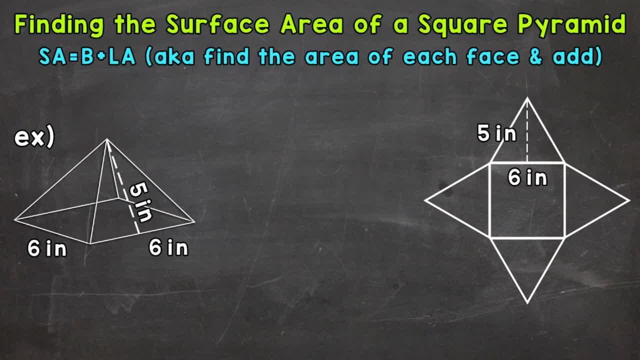 faces. The lateral faces are the triangular faces going around the pyramid, so to speak. We need to find the area of all of these and then add them together to get the total surface area. Now there are a couple of different ways to work through these. 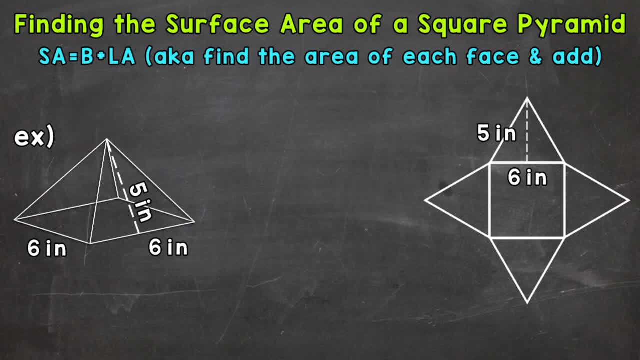 so I'll show you some different options as far as finding the surface area of a square pyramid. So let's jump into our example, where we have a square pyramid with a square pyramid. The square pyramid has a slant height of five inches, and then the sides of the base are six inches. 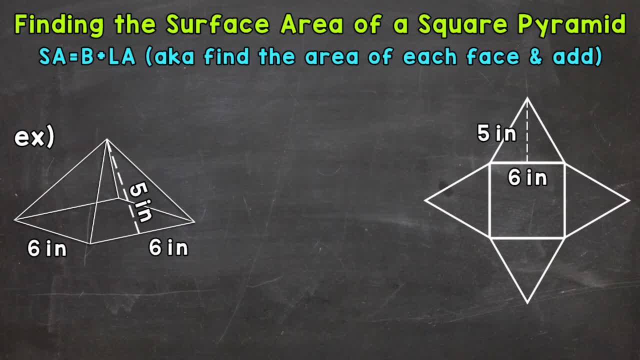 The first thing that I'm going to do is write out: surface area equals the area of the base plus the lateral area. That's going to get us started. Then we'll plug in our information. Let's use the net on the right of the screen to help us do this. You can think of 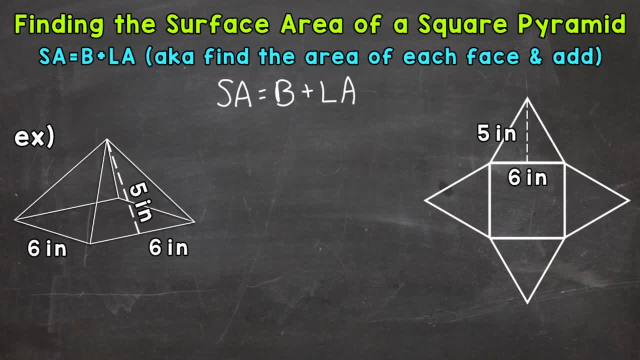 a net as an unfolded 3D shape. It shows us all of the parts, so to speak. So we're going to start with the area of the base. Now for this square pyramid, the base is six inches by six inches And we can see on our net: we have six inches, and then all of the other sides are six inches as well. 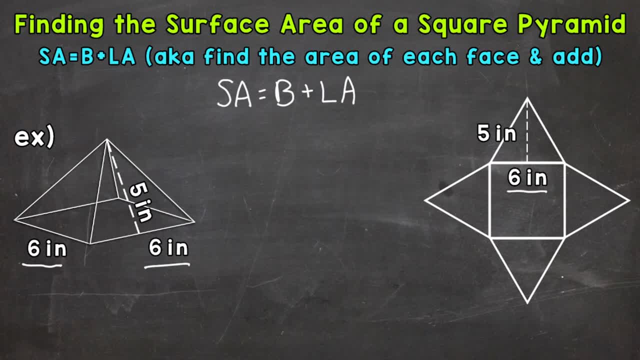 So to calculate the area of a square we can do, I'm going to come to the right here and show some work. One of the sides squared And we know that we have six inch sides, so let's plug in six And six squared means six times six, So the area of the base is 36. 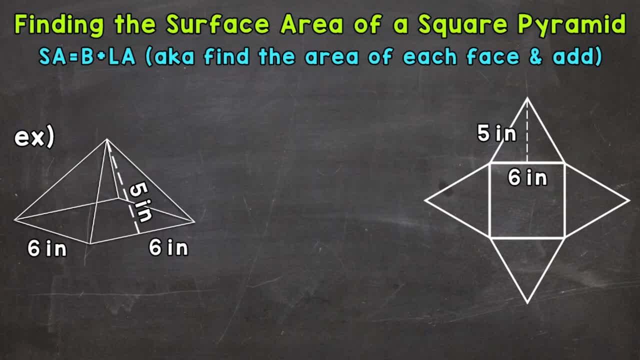 The lateral faces are the triangular faces going around the pyramid, so to speak. We need to find the area of all of these and then add them together to get the total surface area. Now there are a couple of different ways to work through these, so I'll show you some different. 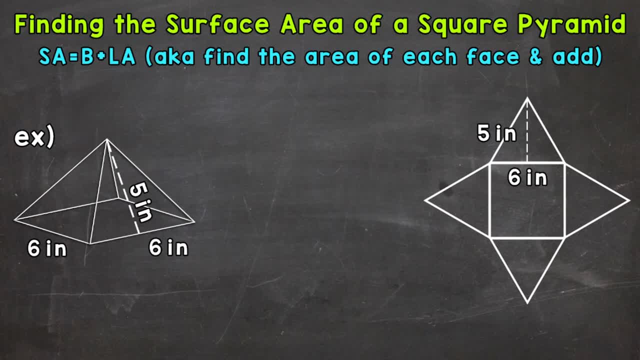 options as far as finding the surface area of a square pyramid. So let's jump into our example, where we have a square pyramid with a slant height of five inches and then the sides of the base are six inches. The first thing that I'm going to do, 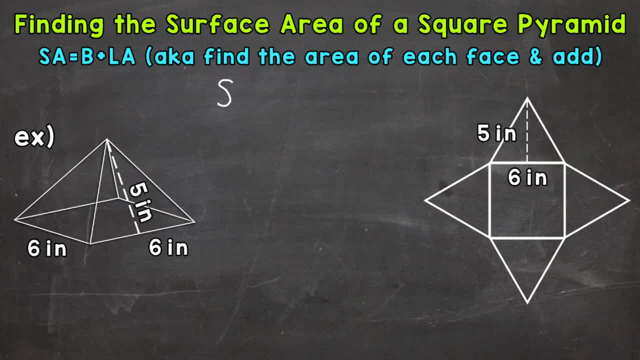 is write out: surface area equals the area of the base plus the lateral area. That's going to get us started. Then we'll plug in our information. Let's use the net on the right of the screen to help us do this. You can think of a net as an. 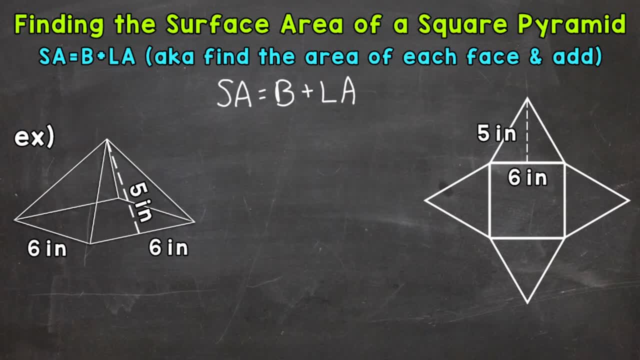 unfolded 3D shape. It shows us all of the parts, so to speak. So we're going to start with the area of the base. Now for this square pyramid. the base is six inches by six inches and we can see. 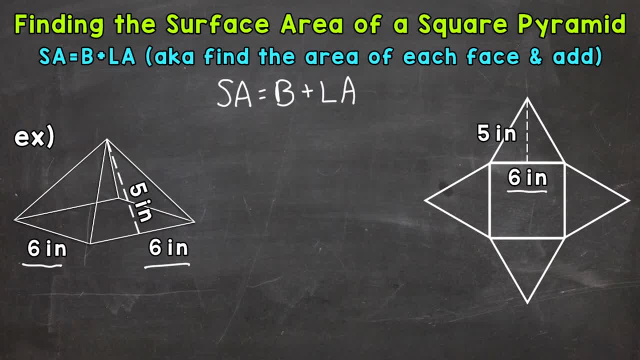 on our net we have six inches, and then all of the other sides are six inches as well. So to calculate the area of a square, we can do. I'm going to come to the right here and show some work. one of the things that you can do is to look at our map. This is a square pyramid and we have a square. 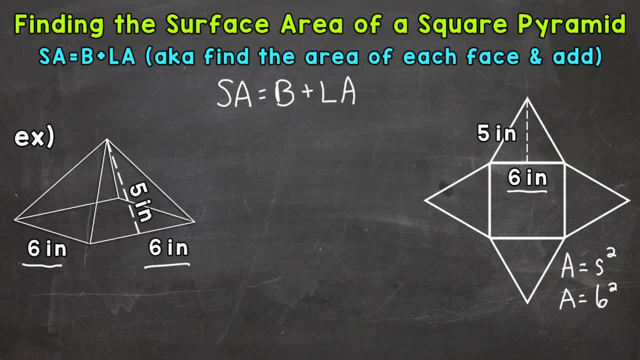 pyramid, And it's a square pyramid. Now you can tell that our base is six inches by six inches, So we're going to use the area of the base as a square. So let's plug in six and six squared means six times six, So the area of the base is 36 square inches. So let's put that in to our net. 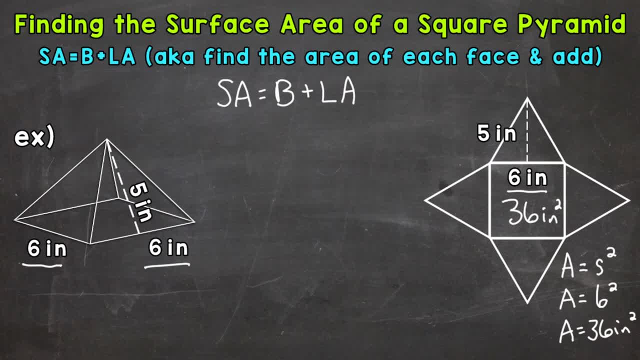 here And now we'll find the area of all of our lateral faces. the bases sides are all the same, so we just need to find the area of one of the triangular lateral faces and we will have the area of all of them, because they are all the same. so we can use the 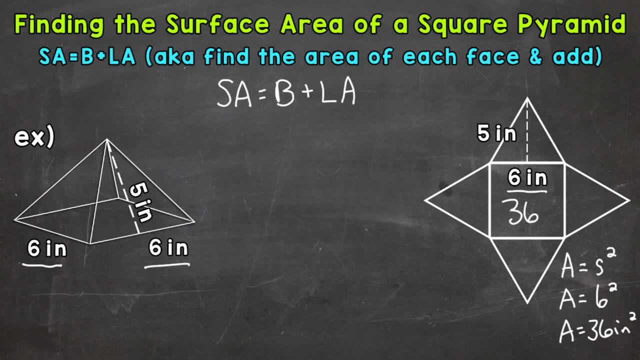 square inches, So let's put that in to our net. here And now, we'll find the area of all of our lateral faces And since this is a square pyramid, that means it's a regular square pyramid, So we're going to plug in the area of the base. 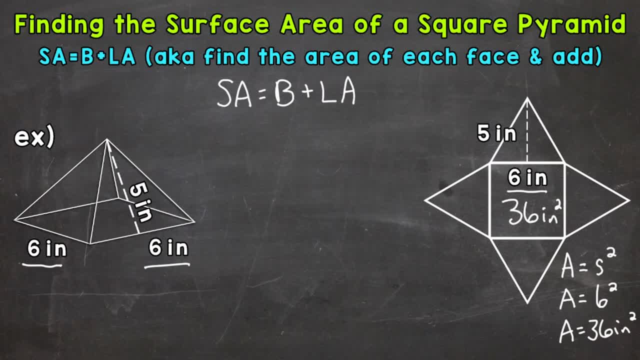 And since this is a regular square pyramid, that means it's a regular square pyramid, Meaning the base's sides are all the same. So we just need to find the area of one of the triangular lateral faces And we will have the area of all of them, because they are all the same. 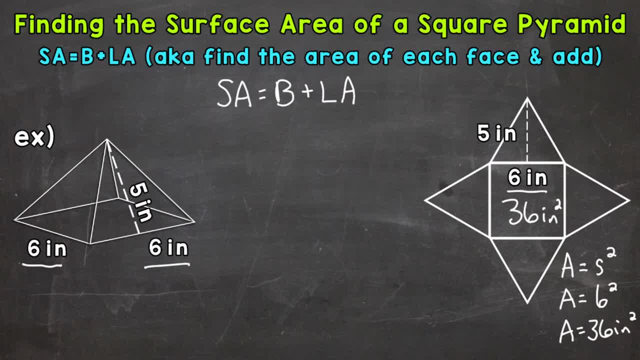 So we can use the formula: area equals one half times base times height. So area equals one half times base times height. Now you can also use base times height divided by two, Multiplying by half or dividing by two. same thing, Whatever formula you like to use, for the area of a triangle. 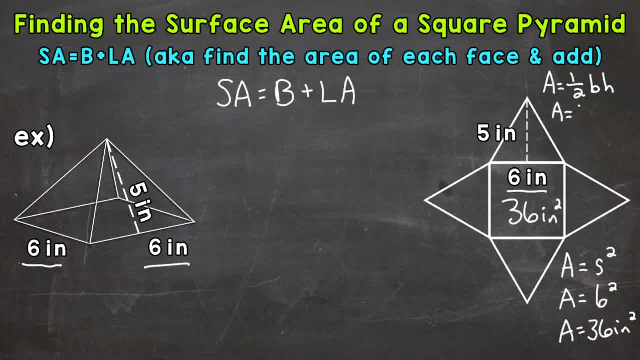 Now we plug in, So area equals one half. Well, the base of this triangle is six inches, So let's plug in six times the height of five inches. So six times five is 30. So we end up with one half Times 30. And we will squeeze this in, So the area is 15 square inches for each of our. 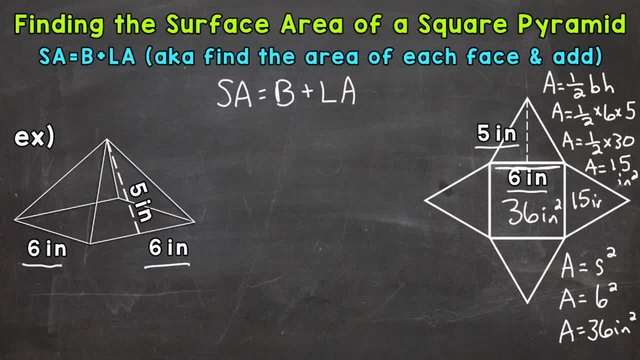 lateral faces. So let's put that in here: 15 square inches for each of these. Now that we have the area of each face, we can add everything to get the total surface area. So let's plug it all in and calculate here. 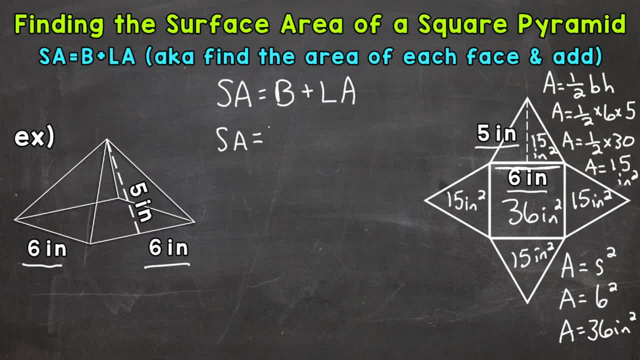 So the area of the base was 36 square inches, So let's put in 36 for the area of our base. Plus we need the lateral area, So all of the triangular lateral faces. So each had an area of 15 square inches, So we need four 15s here. 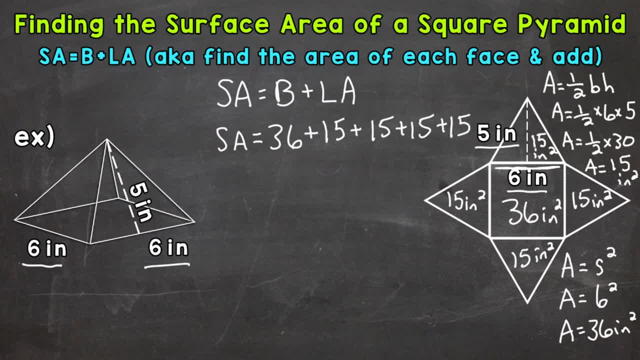 And then we'll add everything to get our total surface area. So we have four 15s, So 15 times four, or 15 plus 15 plus 15 plus 15.. Either way it's going to give us 60. So let's break this down and we'll end up with 36 plus 60. And again, that 60 is coming from. 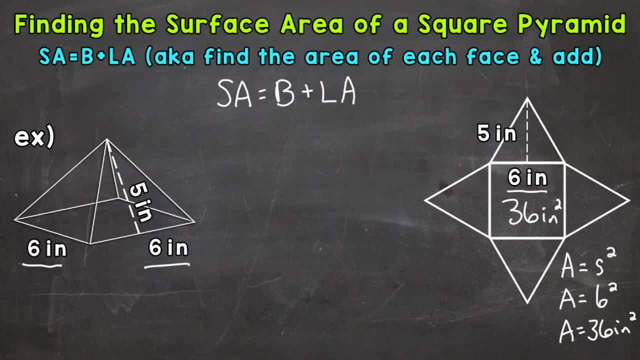 formula: area equals one half times base times height. so area equals one half times base times height. now you can also use base times height divided by two, multiplying by a half or dividing by two. same thing, whatever formula you like to use for the area of a triangle. now we plug in. 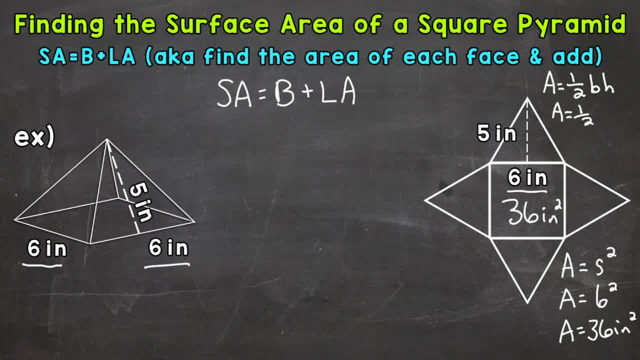 so area equals one half, while the base of this triangle is six inches. so let's plug in six times the height of five inches. so six times five is thirty. so we end up with one half times thirty and we will squeeze this in, so the area is 15 square. 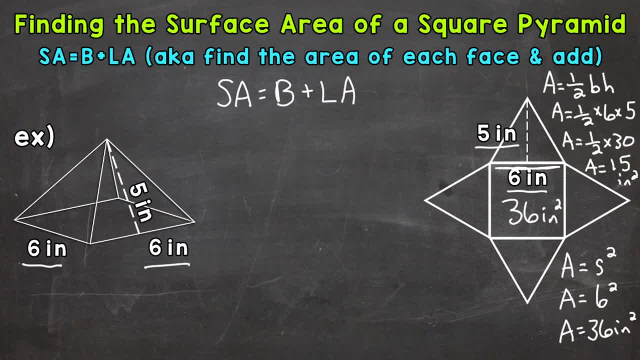 inches for each of our lateral faces. so let's put that in here: 15 square inches for each of these. now that we have the area of the triangle of each face, we can add everything to get the total surface area. so let's plug it all in. 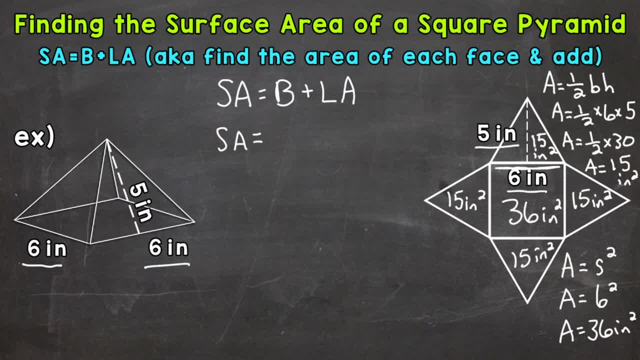 and calculate here. so the area of the base was 36 square inches. so let's put in 36 for the area of our base, plus we need the lateral area, so all of the triangular lateral faces. so each had an area of 15 square inches. so we need 4 15s here. 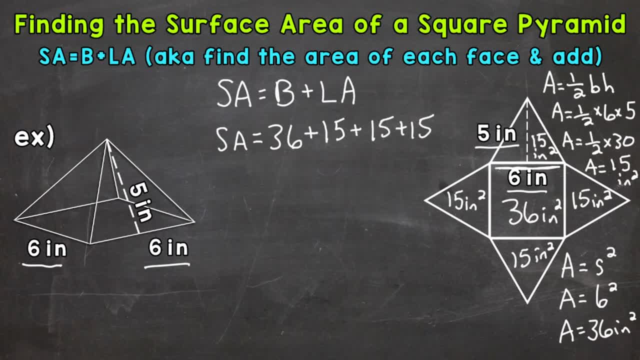 and then we'll add everything to get our total surface area. so we have four fab's. so fifteen times four, or 15 plus 15 plus 15 plus 15. either way it's going to give us 60. so let's break this down and we'll end up with 36 plus 60. and again, that 60 is coming from those 4 15s. so i 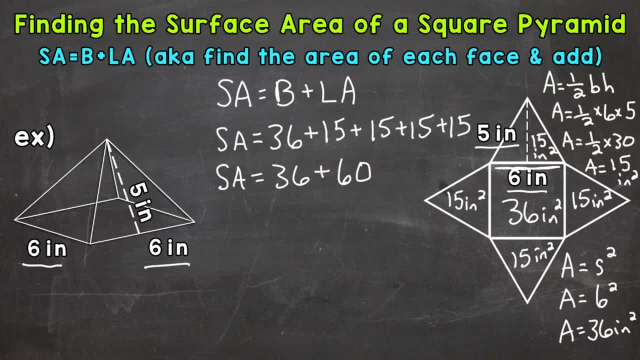 added those four 15s together from her, so we have four square inches and then we need six, in case we need together first, or you can do 15 times 4 and, to wrap it up, 36 plus 60 is going to give us a total surface area of 96 square inches and that's our final. 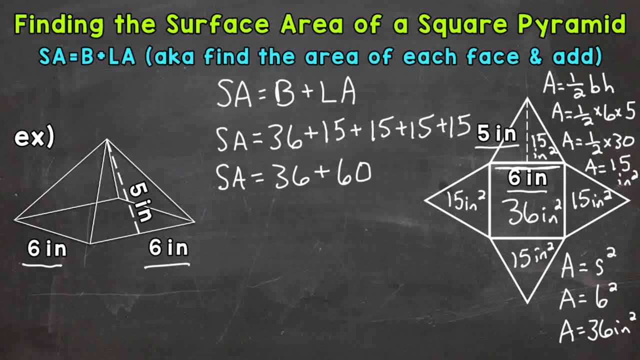 those four 15s. So I added those four 15s together first, Or you can do 15 times 60. So it's going to give us 36 plus 60. And to wrap it up, 36 plus 60 is going to give us a total surface. 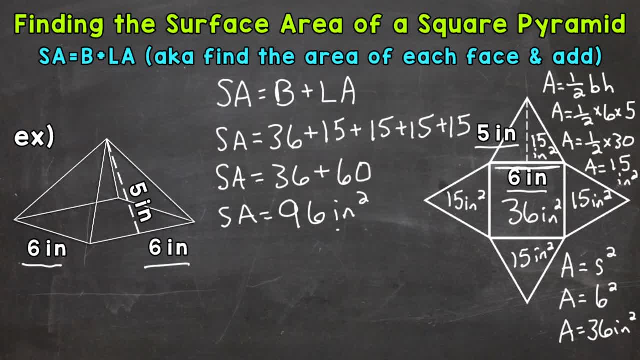 area of 96 square inches. And that's our final answer. Now I would like to show you one other way we can solve. to find the surface area of a square pyramid, We can use the formula: surface area equals the area of the base plus one half. 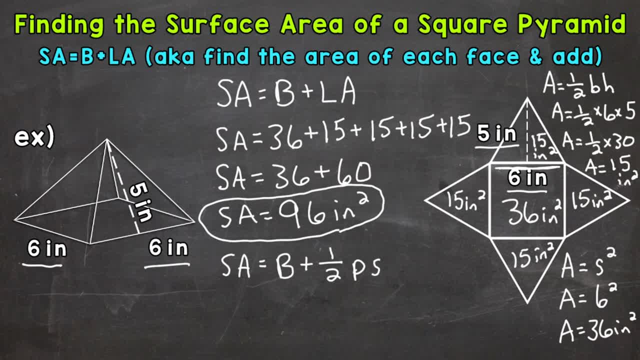 p and then s, Where the p stands for the perimeter of the base and the s stands for the slant height. Now I do want to mention that an l can be used to represent slant height as well. You'll see both, but it doesn't matter which. They mean the same thing, Now that we have our formula written out. 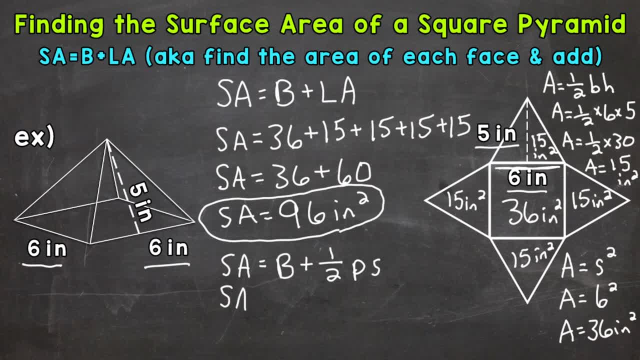 we can plug in. So surface area equals well the area of the base plus one half of the base. We've already calculated that It was 36 plus one half times the perimeter of the base. we need to do six plus six plus six plus six or six times four. 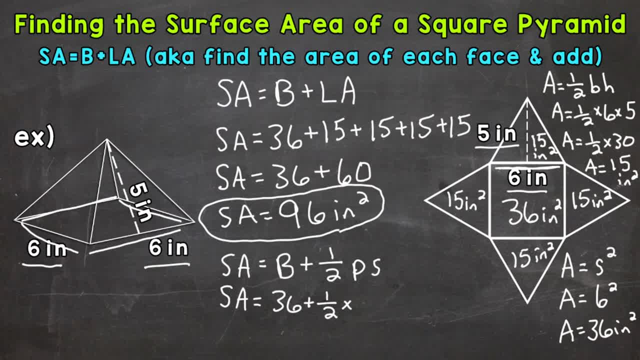 So the perimeter of our base is 24 times the slant height of five inches. right here Here let's also calculate. We know the perimeter of our base here equals 36 as well, Which means that the perimeter of the base we need to do 6 plus and 3 times 4 together so we can look up and see what our pyramid looks like. so far, We have nosso perimetro aqui também 방, as 36 plus 36 plus 6 times 4. 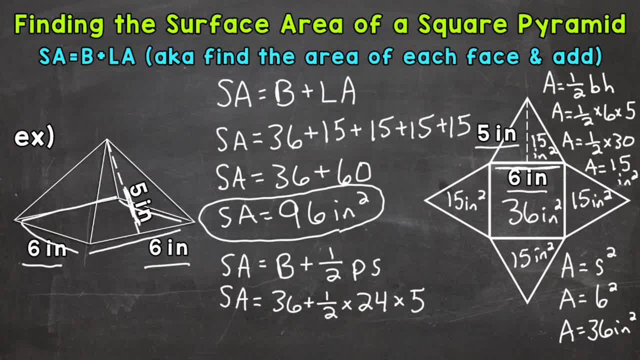 here. Once we have everything plugged in, we can solve, and we can start simplifying or plug this in to a calculator and solve it in one step. I'm going to simplify here. I'm running out of room, but we can make it work. So surface area equals 36 plus one half times 24 times 5.. Well, one half. 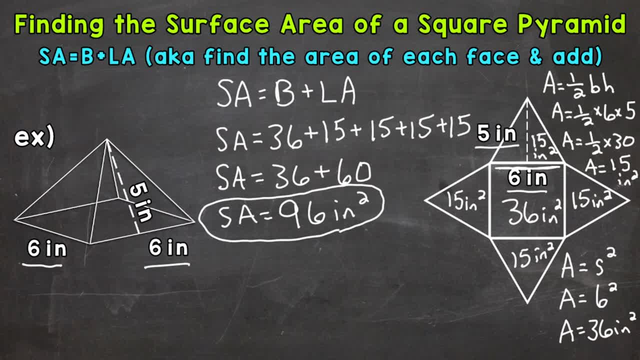 answer. now I would like to show you one other way we can solve. to find the surface area of a square pyramid, we can use the formula: surface area equals the area of the base plus one half P and then S, where the P stands for the perimeter of the base and the S stands for the slant height. now I do want to. 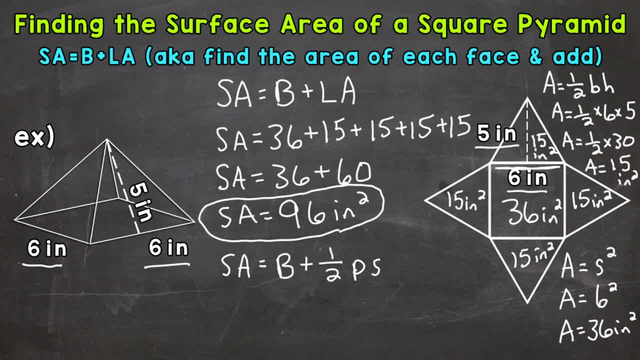 mention that an L can be used to represent slant height as well. you'll see both, but it doesn't matter which. they mean the same thing. now that we have our formula written out, we can plug in. so surface area equals, while the area of the base. we already calculated that it. 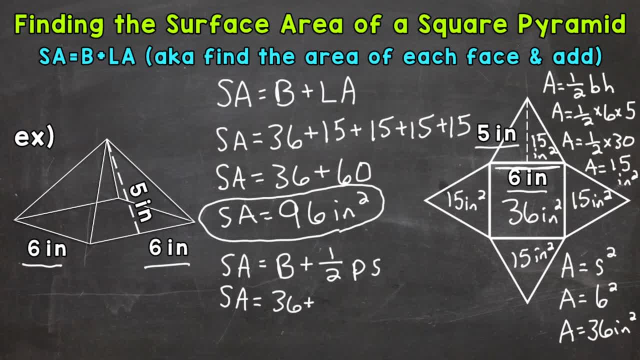 was 36 plus 1 half times the perimeter of the base. we need to do 6 plus 6 plus 6 plus 6, or 6 times 4, so the perimeter of our base is 24 times the slant height of five inches right here, once we have everything. 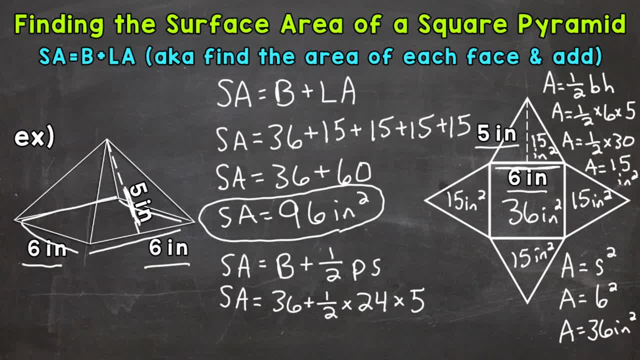 plugged in, we can solve, and we can start simplifying or plug this in to a calculator and solve it in one step. I'm going to simplify here. I'm running out of room, but we can make it work. so surface area equals 36 plus one half. 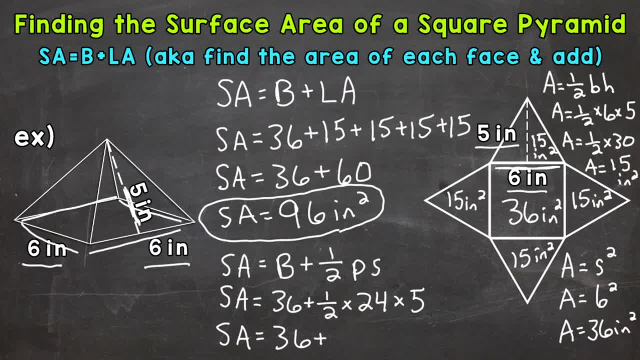 times 24 times 5. well, 1 half times 24 is 37 squared signal. okay, so that means we'll have cross Unternehmen Toe. 12 times 5 gives us 60. So again, I did 1 half times 24.. 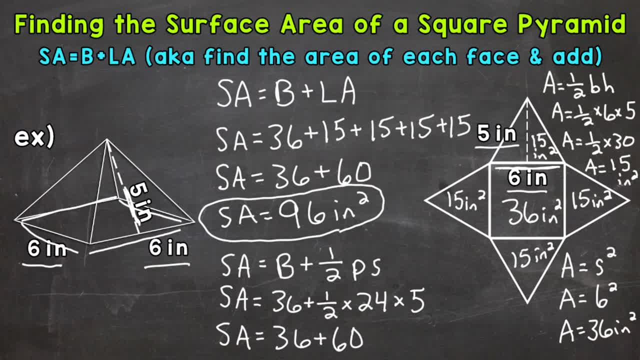 That gives us 12 times 5 is 60. Now we end up with 36 plus 60. And that's going to give us a total surface area of 96 square inches. So we got the same answer as we did up top. 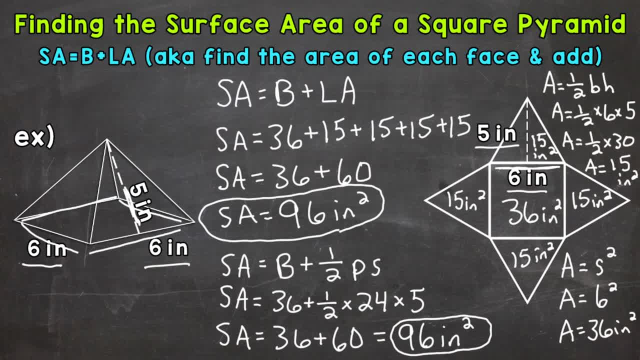 So two different ways there to find the surface area of a square pyramid. We can find the area of each face and add all of those areas together, Or we can use the formula right here: Surface area equals the area of the base plus 1 half times the perimeter of the base, times the slant height.